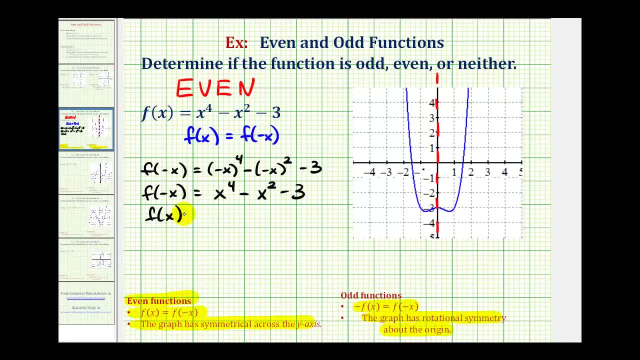 Well notice that f of negative x and f of x are equal to each other. f of x is equal to negative x, f of x is equal to x to the fourth, minus x, squared minus 3.. And therefore, once again, we've shown that the given function is even. 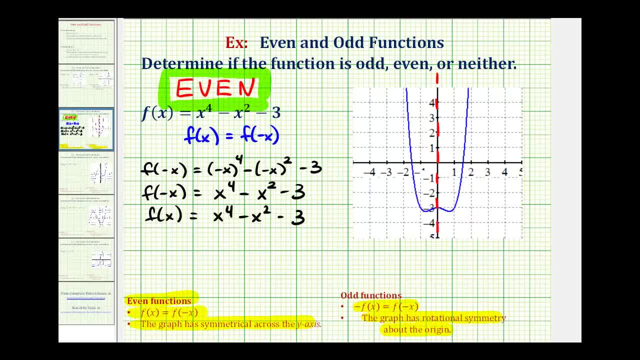 We've shown it graphically, We've also shown it algebraically. And there is one more thing to mention: If we take a look at all the variables on the exponents, and if we had to have a variable on 3, we could write this as 3x to the 0, since x to the 0 is equal to 1.. 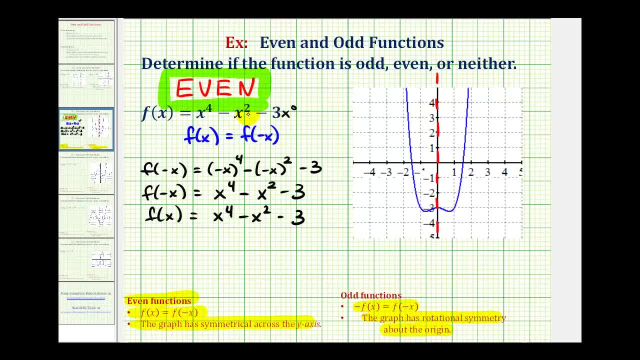 Notice: all the exponents on all the variables are even: 0,, 2, and 4.. So we're going to write this as 3x to the 0, since x to the 0 is equal to 1.. Notice: all the exponents on all the variables are even. 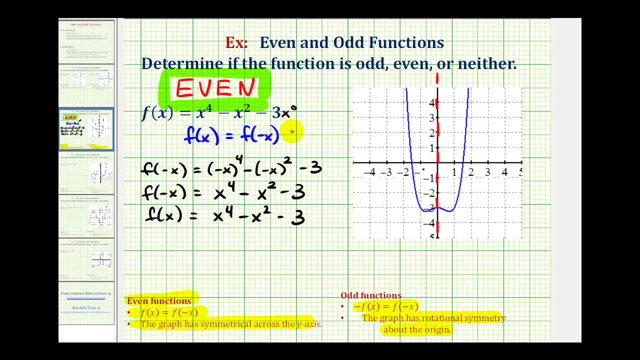 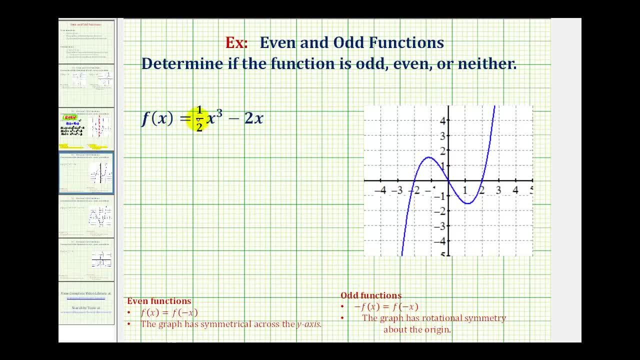 0,, 2, and 4.. And when this is the case, the polynomial function will always be even, which we've already shown. Let's take a look at a second example. Here we have f of x equals 1, half x to the third, minus 2x. 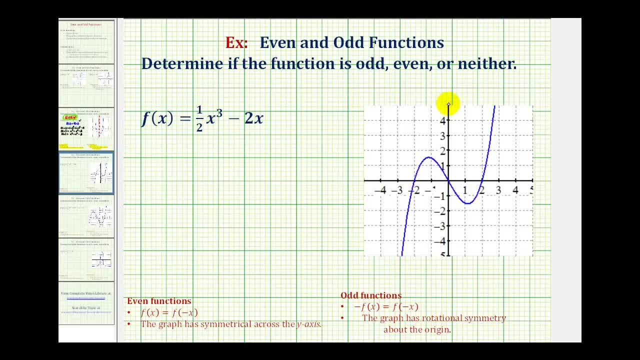 Again, let's start by looking at the graph of the function which, we can quickly see, does not have symmetry about the y axis, but it does have rotational symmetry about the origin, Which means if we rotate this graph about the origin half a turn or 180 degrees. 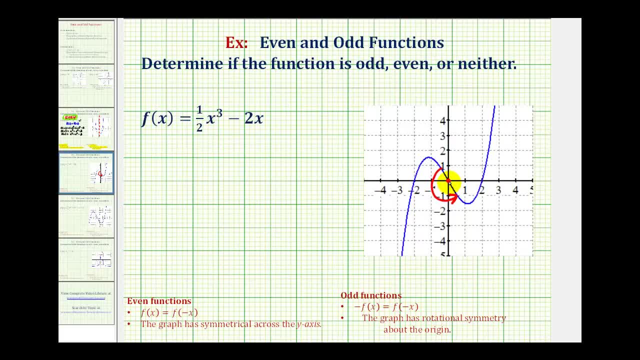 it would remain unchanged. This green half would be where the blue half is and the blue half would be where the green half is. So because of the symmetry about the origin, we know this function is going to be odd. But algebraically we would need to verify that negative f of x is equal to f of negative x. 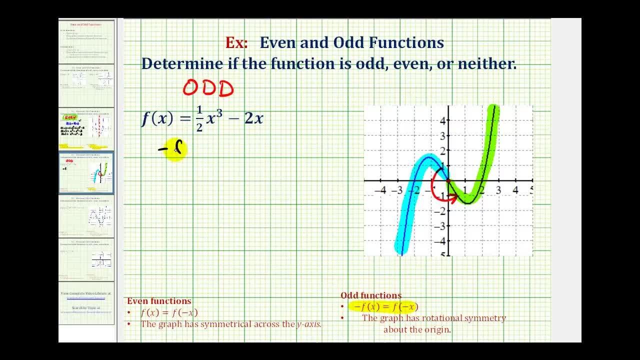 And let's go ahead and do that. We want to show that negative f of x is equal to f of negative x. Let's start with f of negative x. F of negative x will substitute negative x for x in our function. So we'd have 1 half negative x raised to the third, minus 2 times negative x.